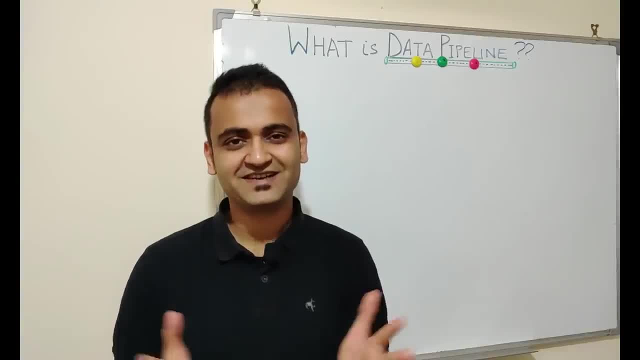 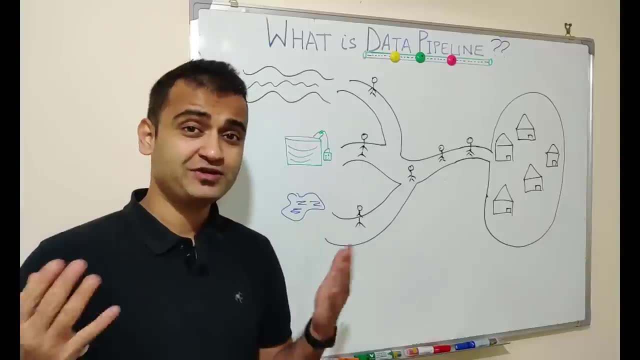 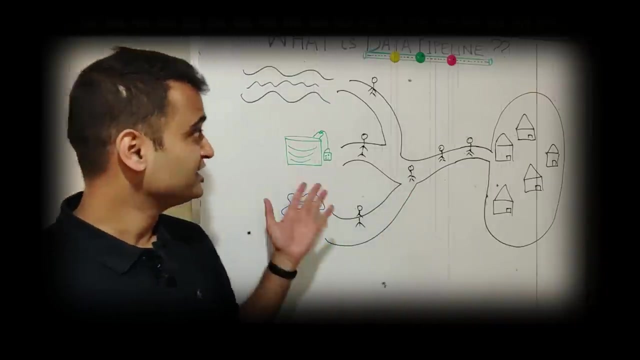 works and what is its underlying architecture? So let's get started. Please subscribe to my channel and hit the bell icon. So yet again, let's start with a layman example. So in good old days, people used to walk miles to fetch water from different natural resources like wells, rivers and ponds. 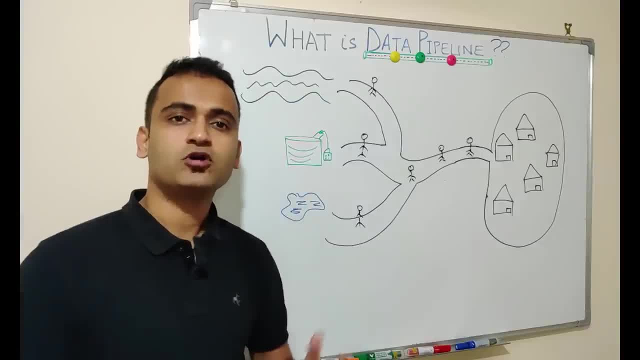 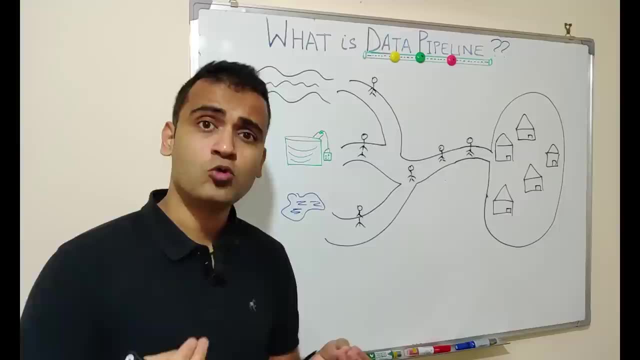 It was a manual process in which people used to fetch the water only for basic needs. But as the human race evolved, our needs also increased with time. We wanted more water, we wanted it automatically, we wanted it frequently and we wanted it frequently. So let's get started. 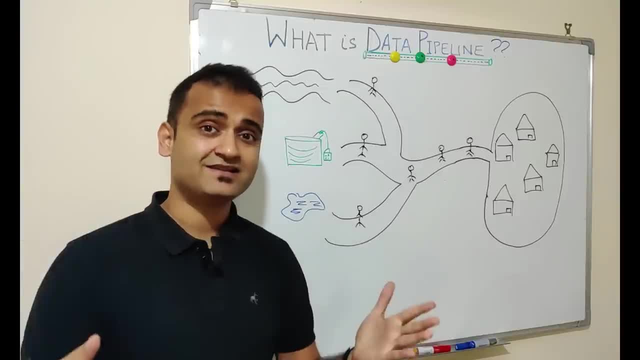 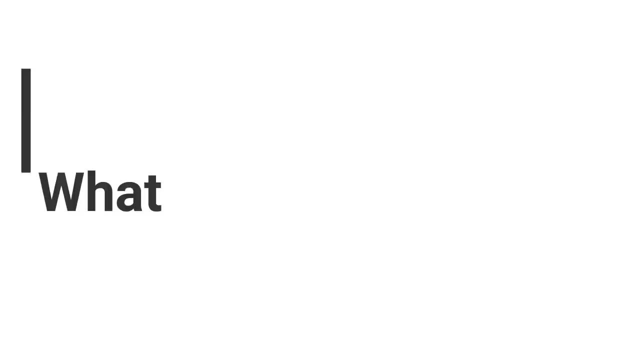 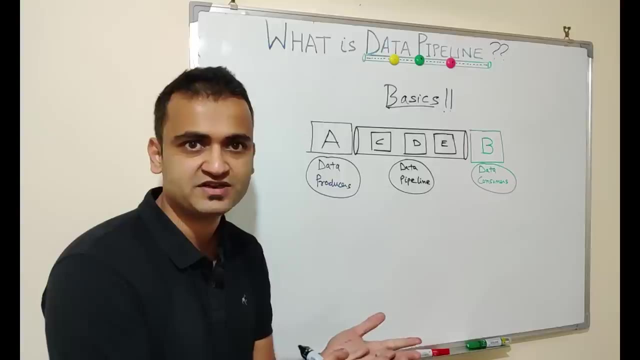 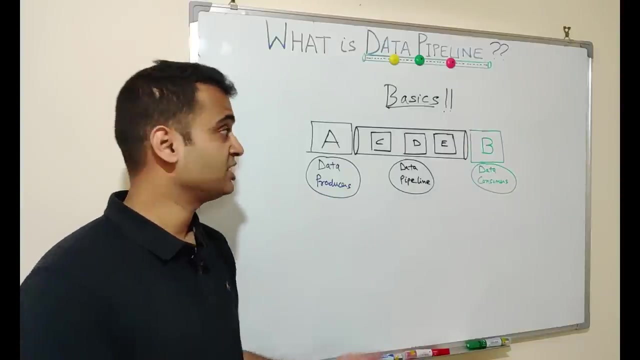 So, friends, basically data pipeline is no different from our traditional water pipeline, which we just discussed. It is a mechanism to transfer data from point A to point B through some intermediary steps like point C, D and E. So these are the points where actual data 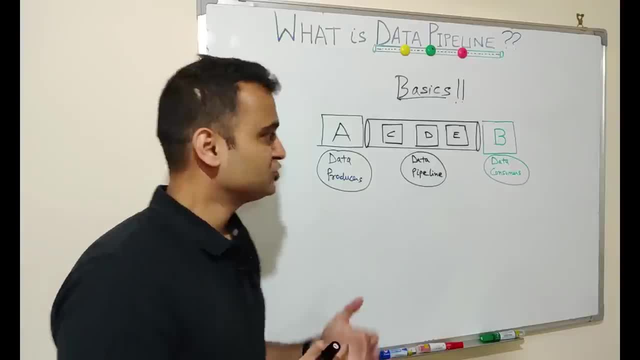 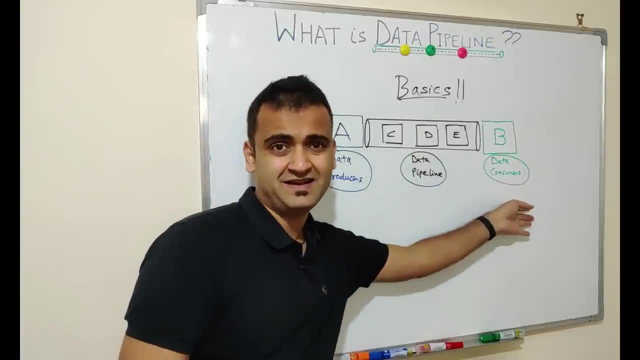 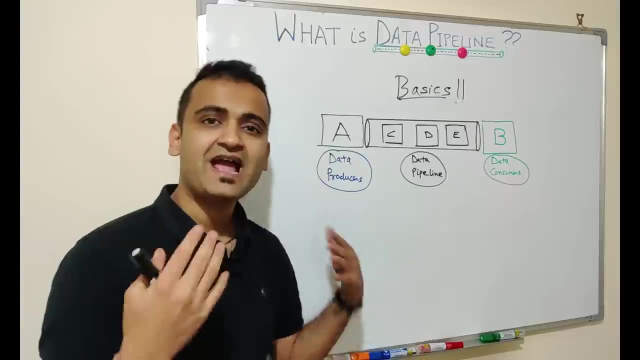 pipelines are used. So let's get started. So in this basic diagram, point A is called as data producer, point B is data consumer, while these points- point C, D and E- are actual data pipeline. So this is a basic diagram. 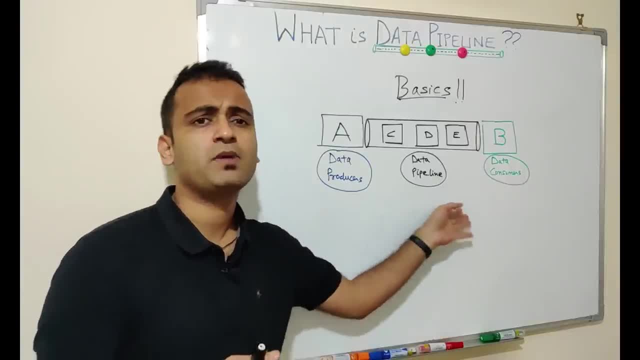 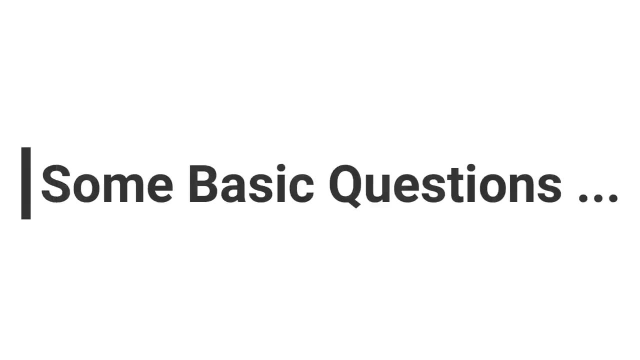 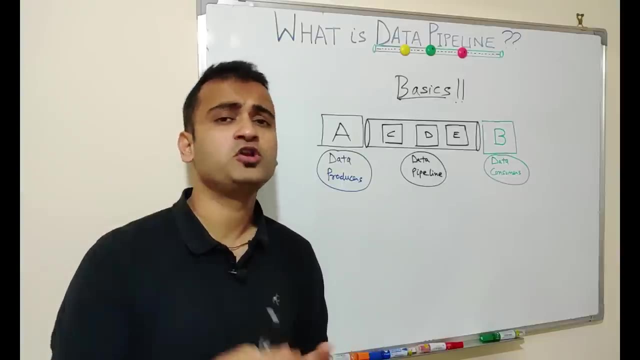 explaining in a very layman understanding how a data pipeline works. But there could be very obvious questions coming into your mind. So the very first question could be why you need data pipeline at the first place. So it basically depends on your requirement In. 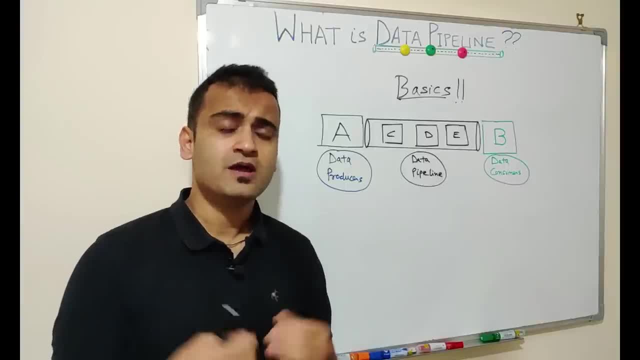 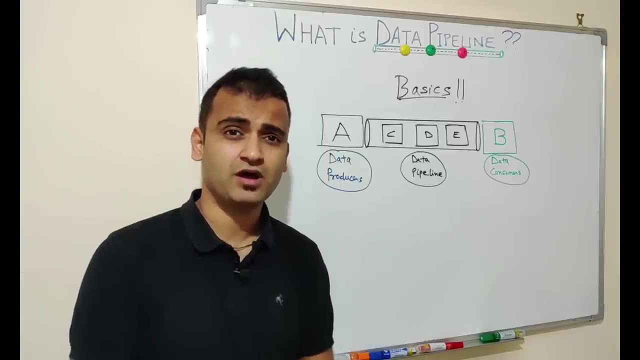 initial days, when this whole technology was still evolving, people used to work on R's to generate a simple report in Excel. People used to store multiple thousands of files in their Windows drive and then process this, And it was a very tedious process. But as the data grew, so did the 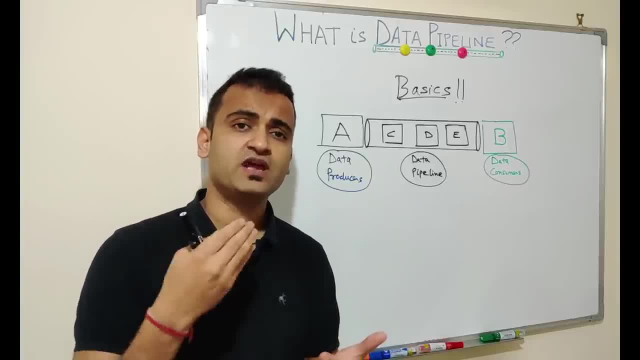 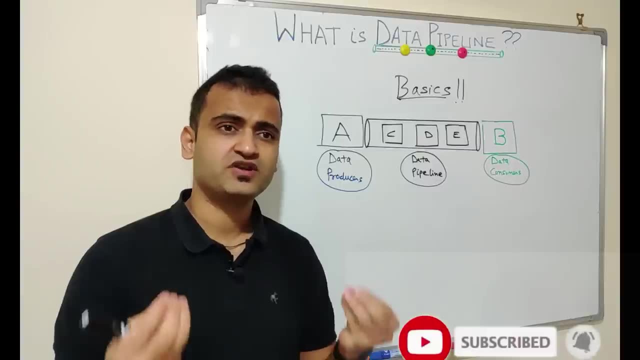 technology, And then we came up with the concepts like data warehouse. we came up with the products- ETL products- which process this data, And then we came up with the concepts like data warehouse, which process this data. But now, today, we have data science coming into picture. we have 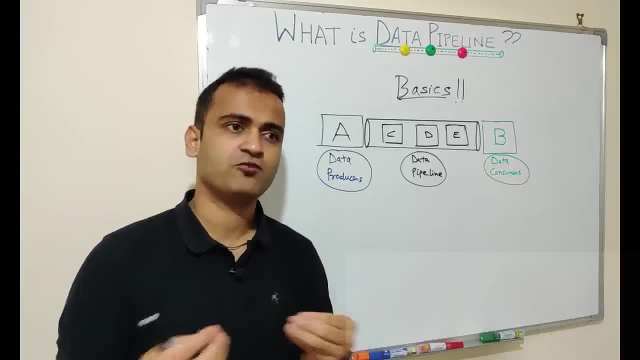 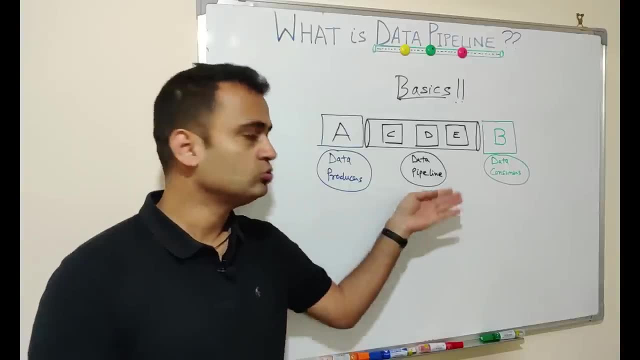 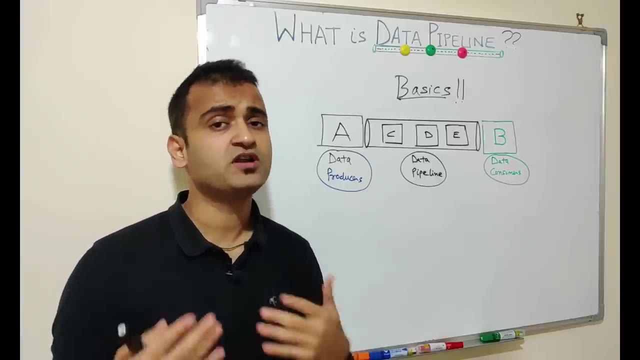 predictive analysis, we do machine learning, AI, everything And for everything. you need good quality data And how you can do it. you can do it by processing it through a data pipeline, But what kind of pipeline you need basically depends on your business need: whether you want it for a 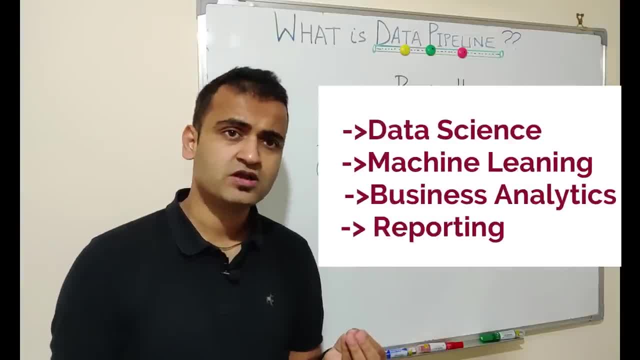 data science project. you want it to build some machine learning models. you want to do a simple business analytics operational reporting- what you exactly want to do. you want to do a simple business analytics operational reporting. what you exactly want will decide what kind of data. 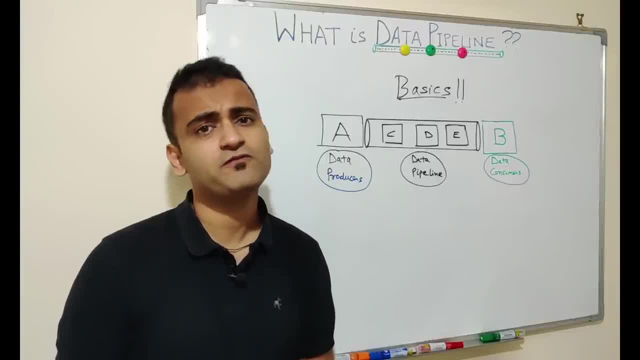 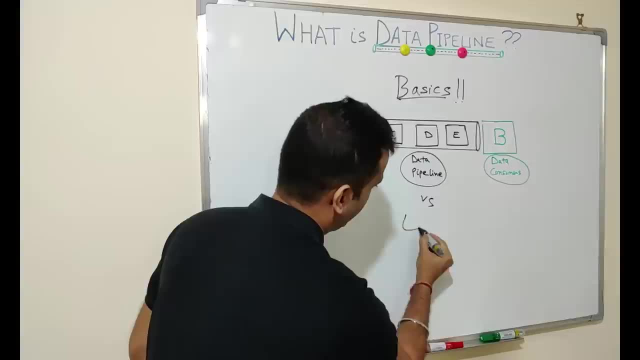 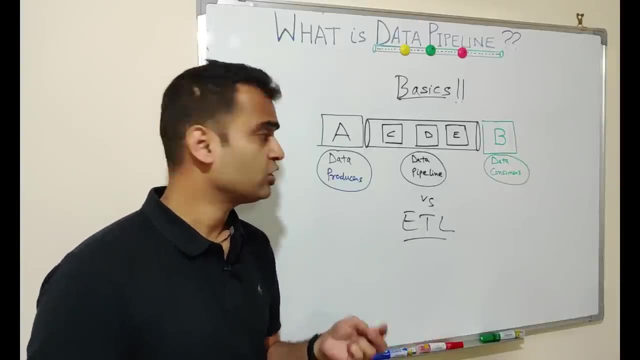 pipeline design, you will go for. A second, very obvious question which might come to your mind is then: what is the difference between a data pipeline and a traditional ETL technology? So this is a valid question, guys, because ETL pretty much does the same thing. then what is the? 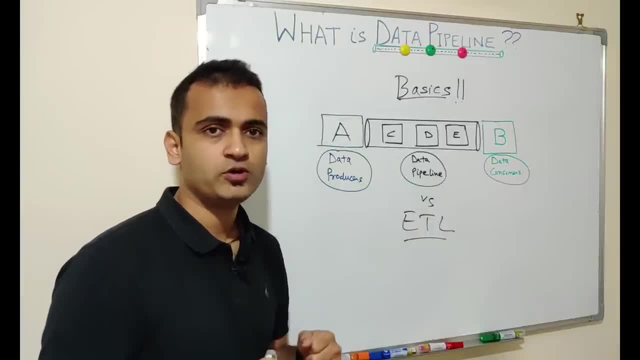 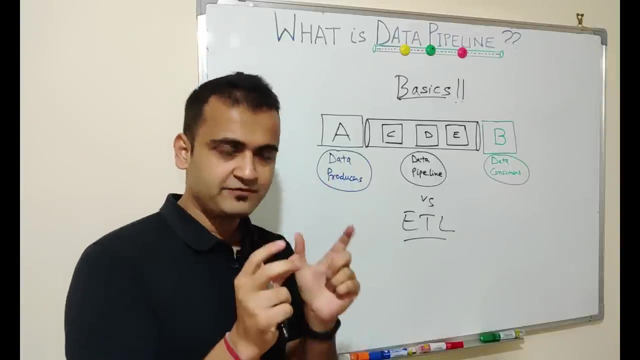 difference, Why this new term has come in and become so popular nowadays. Because data pipeline is considered- or you can consider it- as a parent set. under that ETL is a subset. So data pipeline is a broad umbrella under which ETL falls and fills a certain area of a data pipeline mechanism. So we 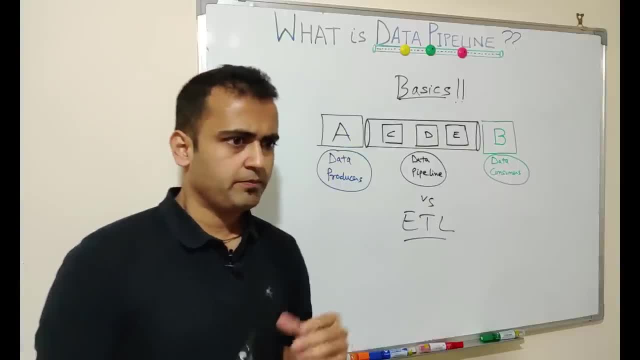 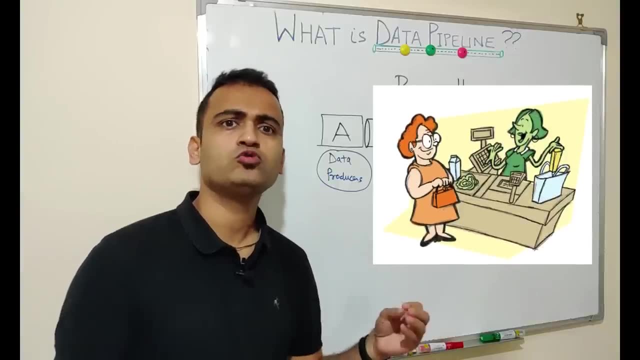 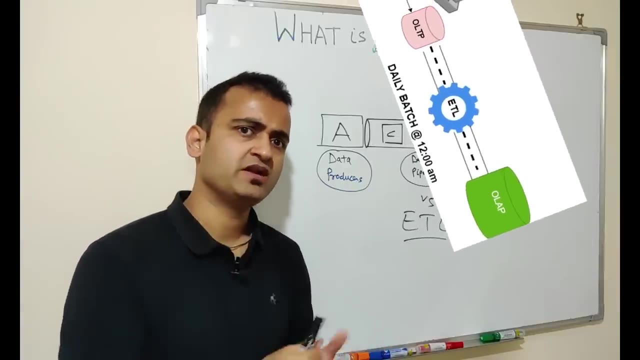 can understand this with an example. So suppose you want to process daily sales data from a point of sale systems from a retail outlet and you want to only do it on a daily basis. So what you will do is you will take the data at 12 midnight from the retail stores, fetch that data, store it in the 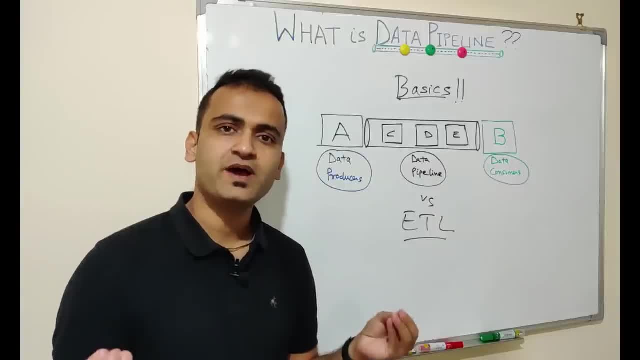 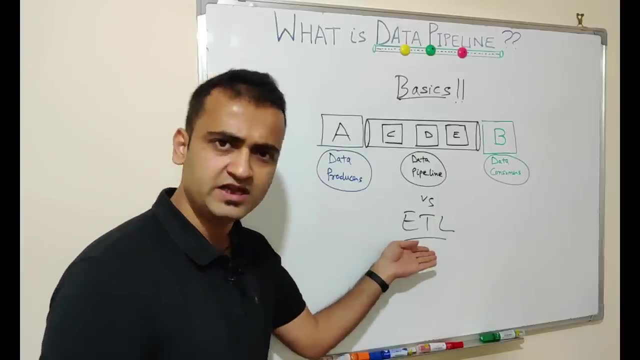 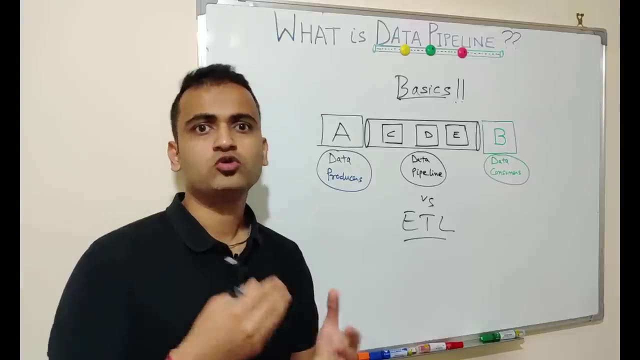 database and then maybe run some reports on top of it. So you are running the batch loads daily And you only need the data to be processed once in a day. This is a perfect case for an ETL design, because you can use any ETL product to do that. But suppose you want again to have 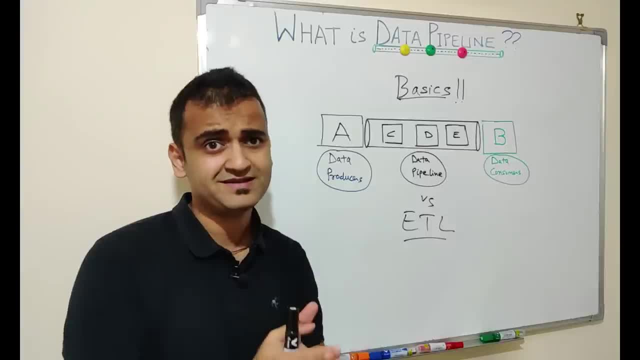 real time data analysis And maybe this time you want to understand what is your product inventory, So you might want to run some real time analytics on your inventory. You want to know how frequently your products are getting replenished in your inventory, how you are capable. 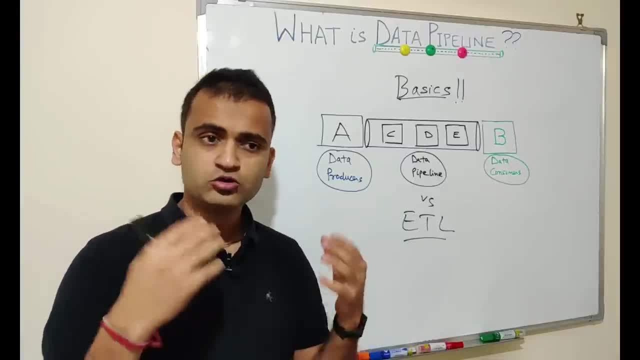 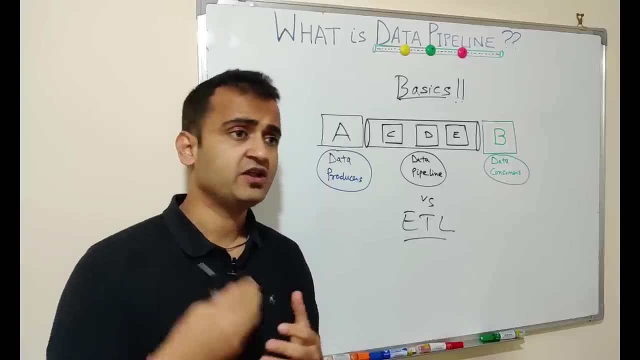 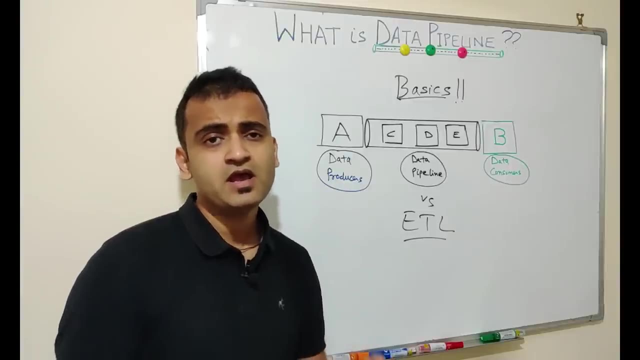 to meet the demand of the customers using your inventory. So in that case you might want to use some sensor data to identify how the stocks are in your current inventory, And you want it maybe every few minutes, maybe every few hours. So in that case you need real time data streaming And 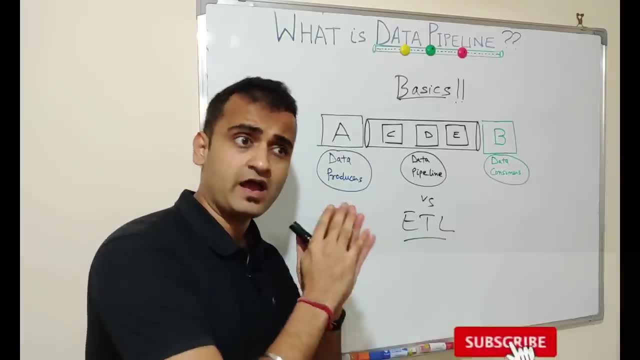 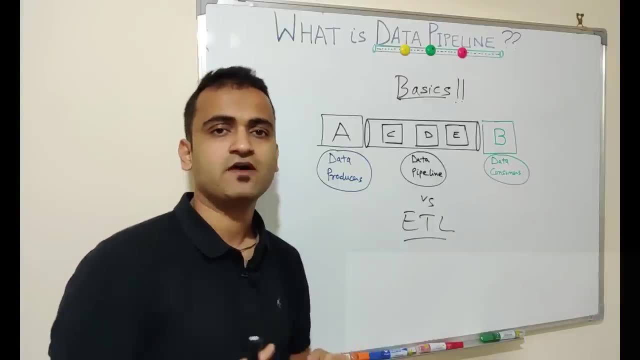 for that there can be a separate, completely new design which might not need or might not work with an ETL technology. you might need real time processing, maybe using Apache, Kafka or some real time message broking service, So in that case you have a 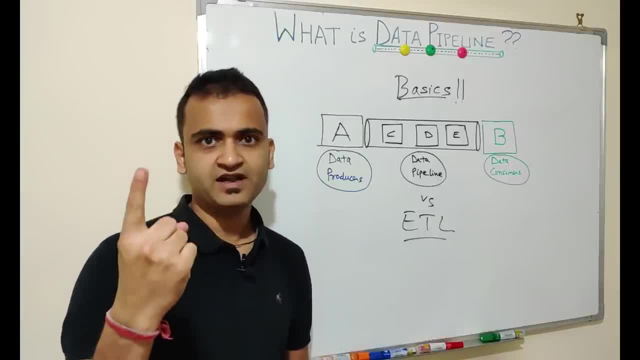 different requirement. So data under data pipeline, you can have real time data streaming and you can have batch data streaming. So these are the two types under data pipeline. But there can be a third type which is called as a lambda architecture. What is a lambda architecture? 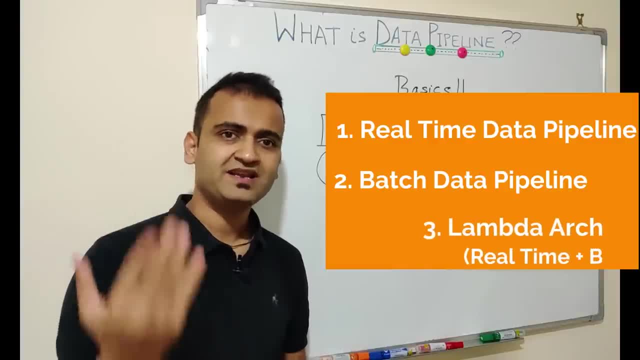 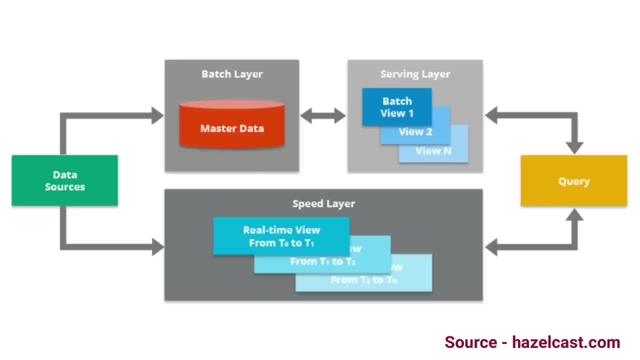 the third type, which is called as a lambda architecture. what is a lambda architecture? which is called as a Lambda architecture? What is a Lambda architecture? Lambda architecture is best of both the worlds. So suppose you want to run both the data pipelines under one umbrella. 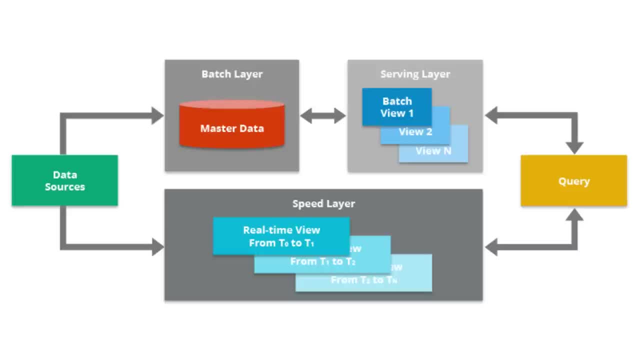 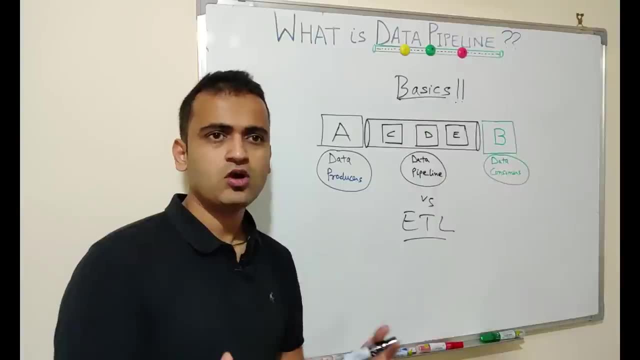 then you can design your data pipeline in that way- and it will be called as Lambda architecture- where you will have your batch data pipeline and you will also have your real time data streaming. So now let's dig deep into the advanced architecture of a data pipeline to get more insight. 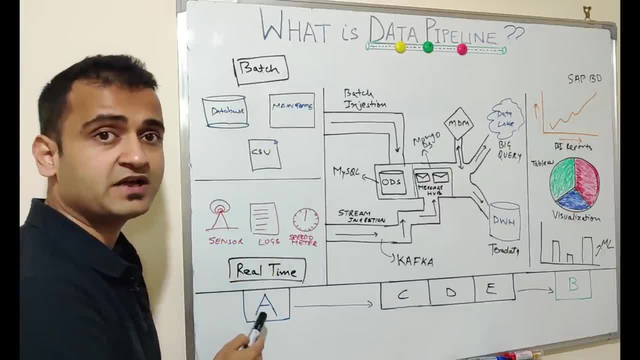 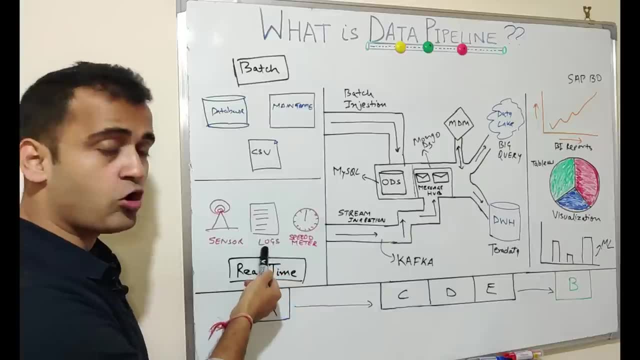 So on the left, we have two types of data getting generated: the batch data, which is on premise, and then these real time data from your sensor, from your log devices and maybe your speedometer. So all these are coming in real time, maybe through satellites and IoT sensors. 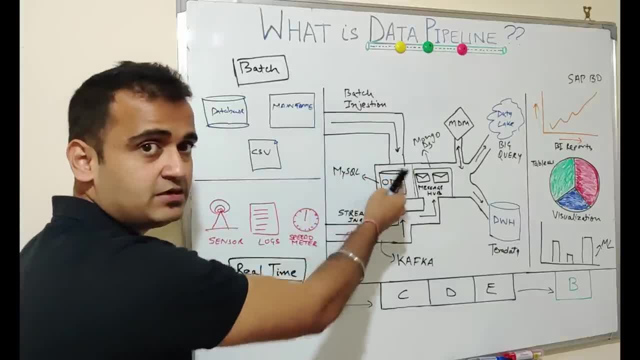 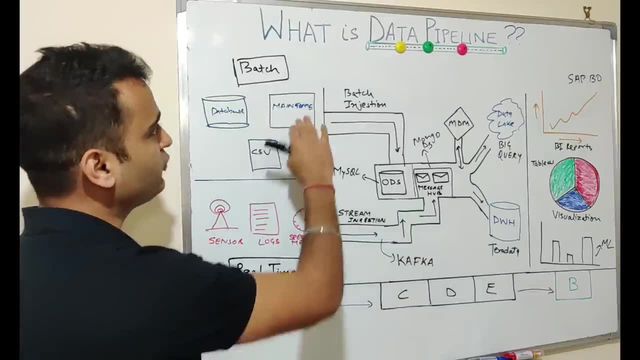 and these are your traditional data. So you will have batch ingestion, batch streaming for this kind of data and you will have real time streaming ingestion using this. So for this you can have a traditional ETL tool like BODS. okay. 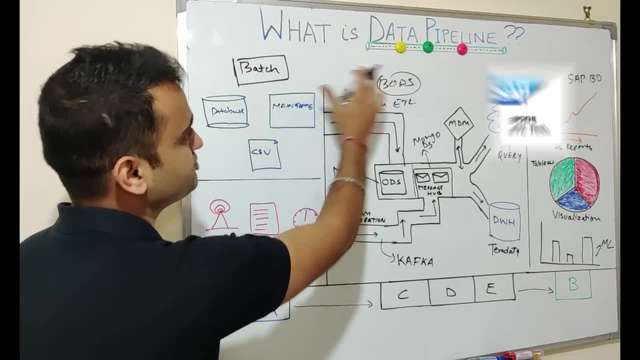 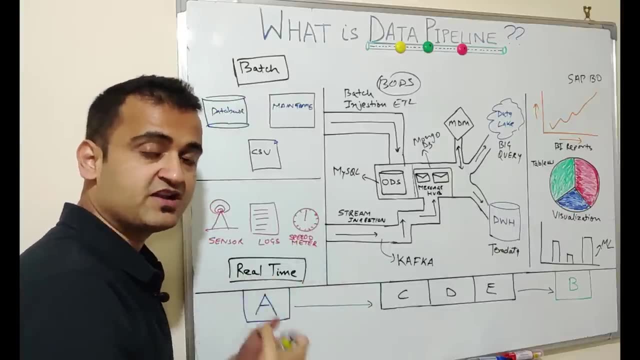 So BODS ETL tool can you know fit into this batch kind of an integration wherein here, for real time, the data is coming in messages? So you need a streaming messages service which is Apache. Kafka can be one of the you know option. 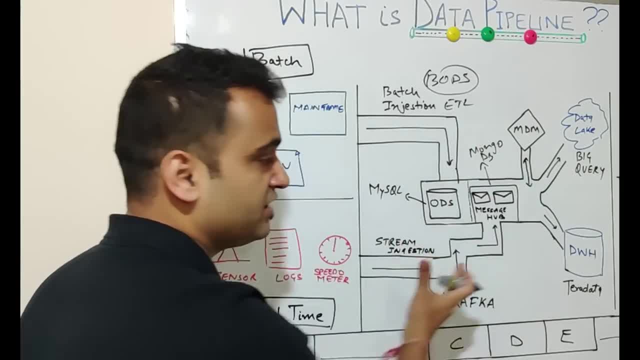 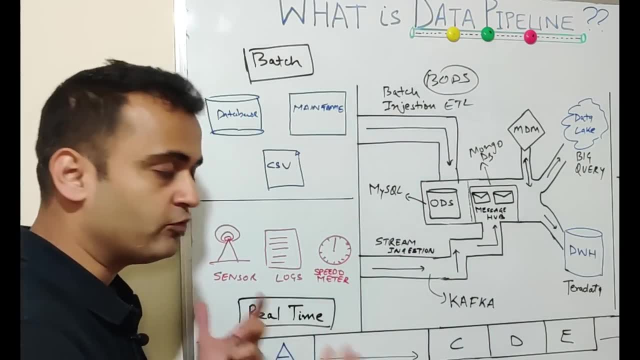 Once you get this data, you will have a central data pipeline which you can see. in this whole design- All the components here- forms your data pipeline, So you can see the overall data pipeline. So maybe your data needs to get stored in your operational data store. 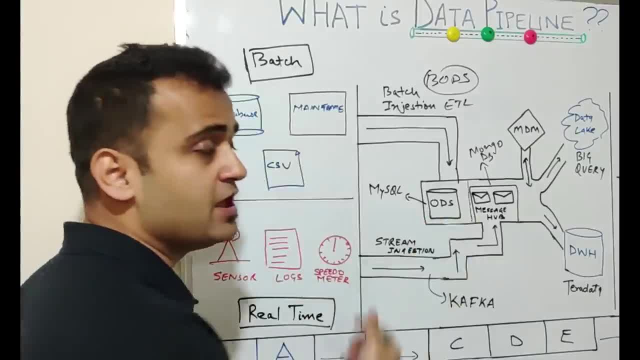 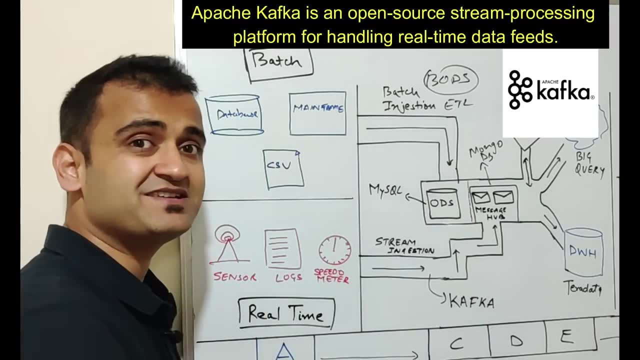 because in a traditional ETL design you have to stage your data, So your ODS layer can stage that data, Whereas in real time you can have your Kafka messages getting streamed and stored in a message hub. It could be a NoSQL database like MongoDB. 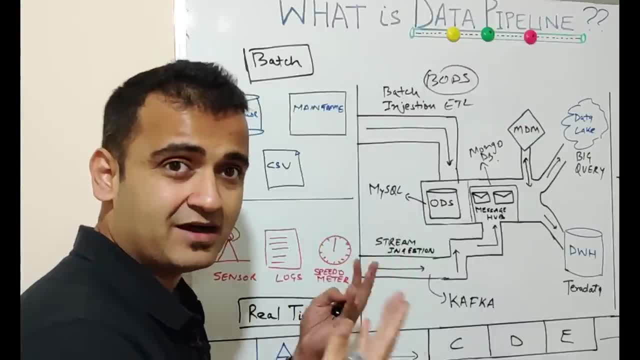 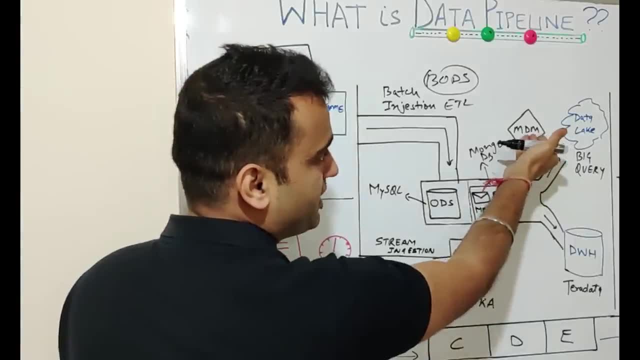 While all this data is coming and getting stored into your staging environment, you can continuously try to enter data, improve the quality of data using master data management, So this MDM process can fit in and continuously see the data which is coming into your pipeline. 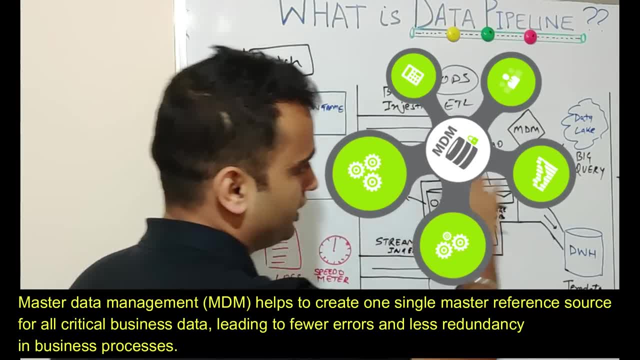 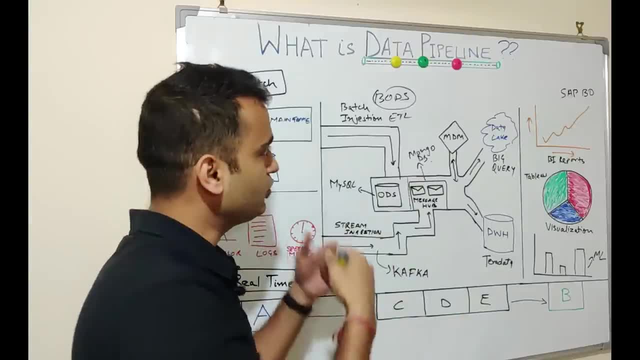 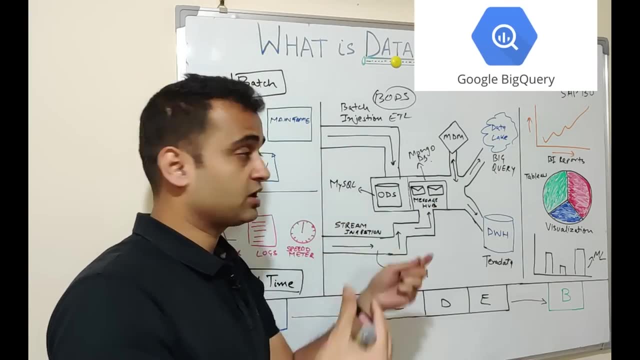 and try to enrich that- the quality of the data in this pipeline. Once this whole data is ready, it can flow into various target streams, So it can go into a data lake. So a possible product could be a Google BigQuery which can store your data on the cloud as a part. 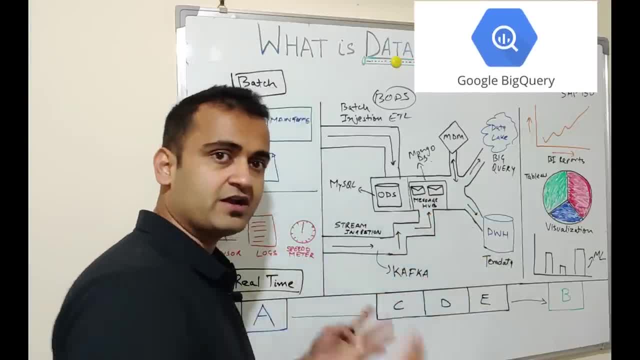 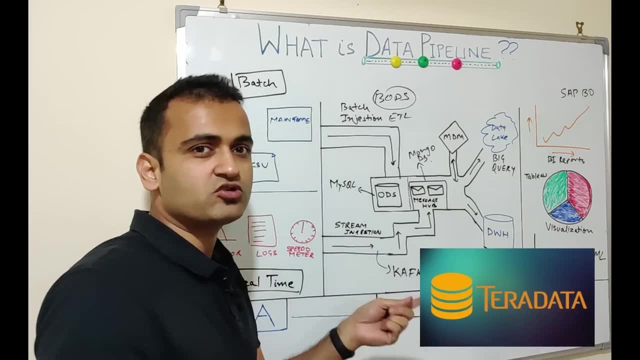 of your data lake solution. You can have your data going into a Teradata data warehouse, So there can be multiple products. So we are not discussing products here, but I'm trying to give you some products so that you get to understand how you can design this whole data pipeline. 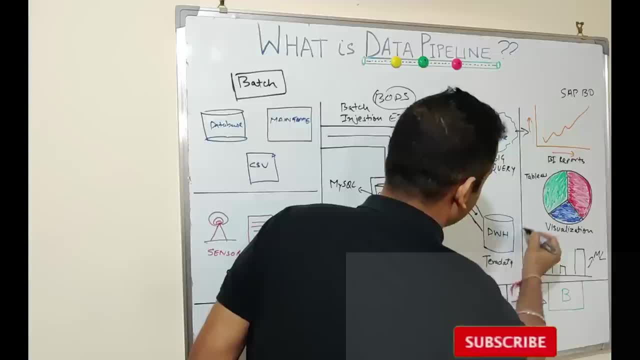 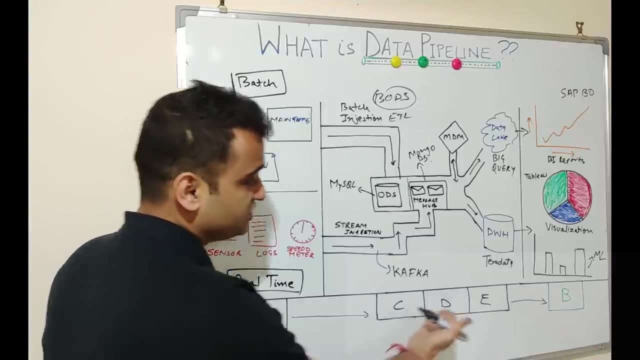 And eventually, once everything is ready, you have data, finally going into point B, which is your last point, where you consume the data. So this is your data producer, This is your data pipeline, And point B, this is your data consumer. 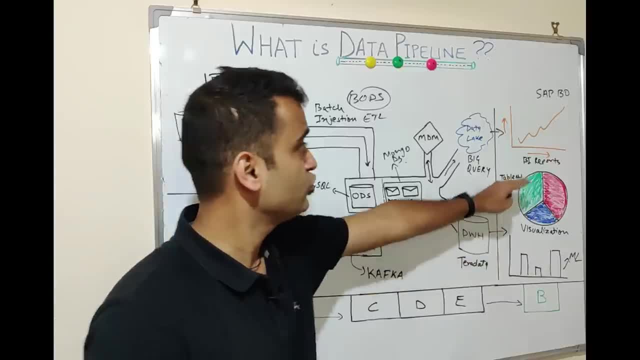 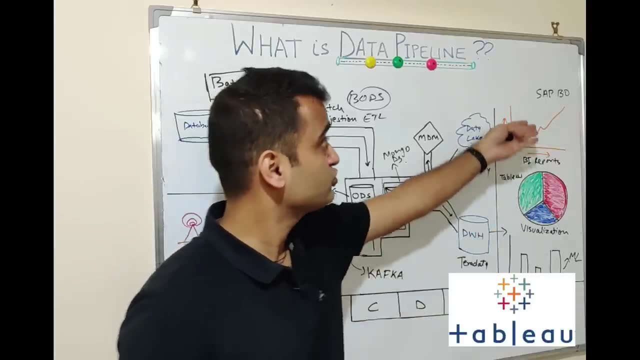 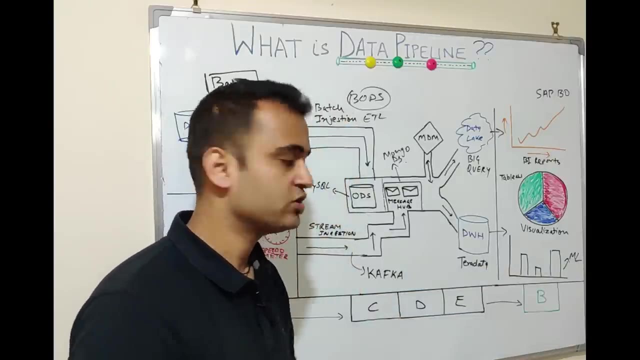 So in the right most end you have the data consumers. So these data consumers could be your BI reports, your operational reports. You can have your visualizations using product like Tableau. Your reports could use SAP Business Objects for reporting And then you can have your ML models to run statistical 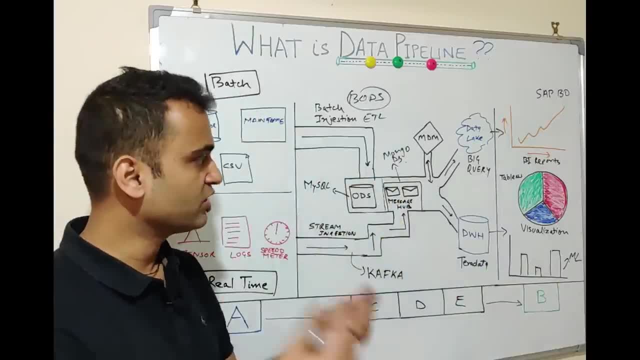 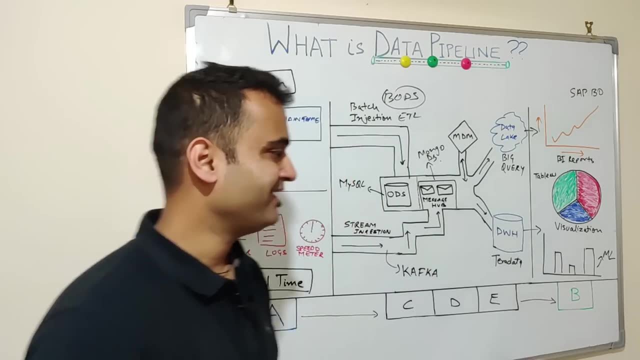 you know data models And you can derive some machine learning algorithms to run on the data which you are getting from your data pipeline. So this whole design is a glimpse of how advanced a data pipeline could be. It could vary, you know, at various places.